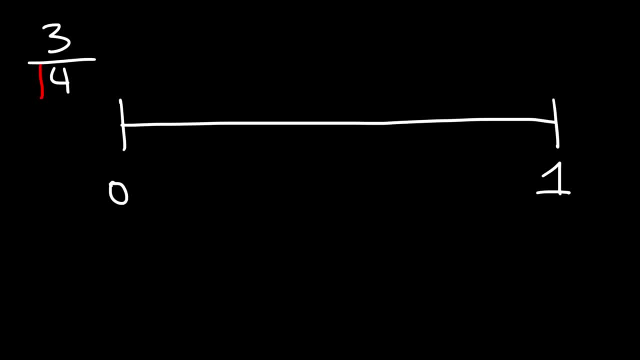 So the first thing you need to do is consider the value of the denominator of the fraction. So it's a four. What that means is you want to break the number line into four equal parts. So I'm going to put a line in the middle and the mark here and here. So this is the first. 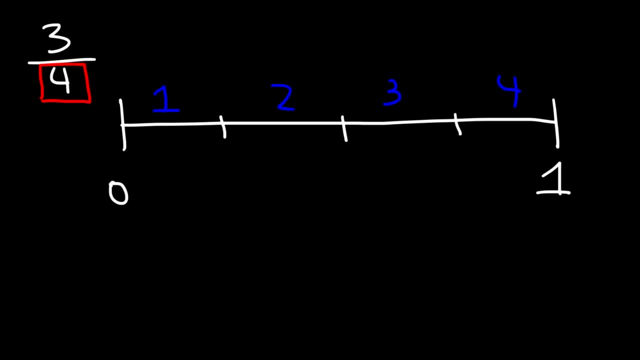 space, second, third and fourth. So there's four equal spaces in this number line between zero to one. Now, at the first mark that's one over four, The second mark is two over four, The third one is three over four, And then the third one is three over four, And this number line here you have to put. 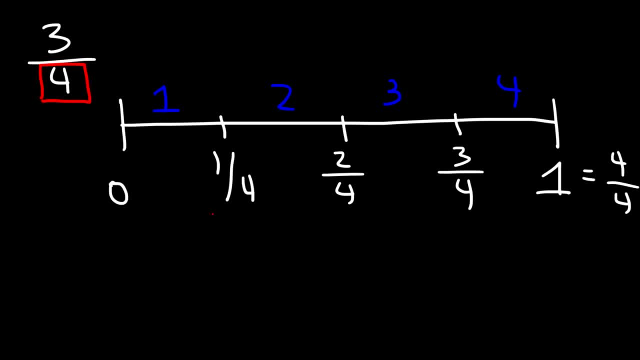 And 1 is the same as 4 over 4.. So 3 over 4 is located right here. It should be placed at the third mark if you break the number line into four spaces. So let's try another example. Where should we place the fraction 4 over 7 along a number line that ranges from 0 to 1 in value? 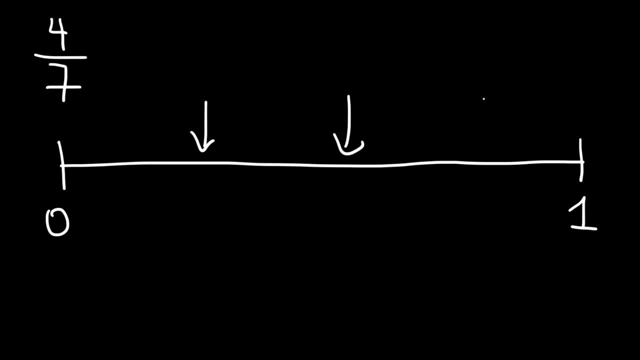 Should we place it here, here or there, Or is it somewhere else? Feel free to pause the video and try that problem. So what we need to do is focus on this number, the 7., And so we need to break up the number line into seven equal spaces. 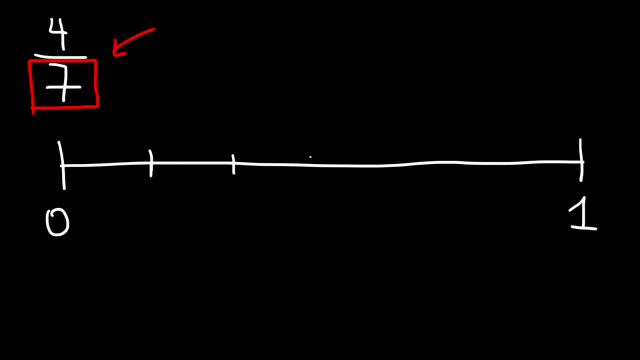 So this is going to be 1,, 2,, 3,, 4,, 5,, 6, and 7.. Now, granted, my trick is to break up the number line into seven equal spaces. The picture on may not be perfect, but you get the picture. 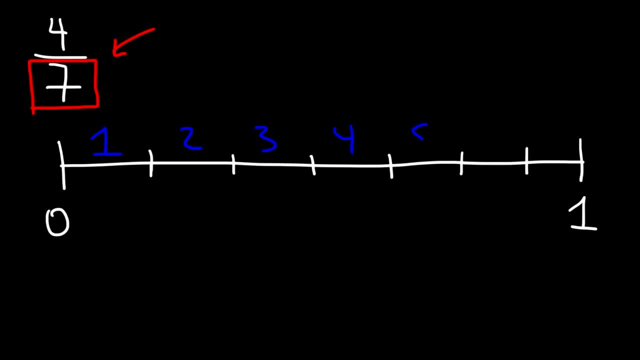 So this is the first space, second, third, fourth, fifth, sixth, seventh. So you want to make seven equal spaces. Now, at the first mark, the value of the fraction is going to be 1 over 7. And then 2 over 7.. 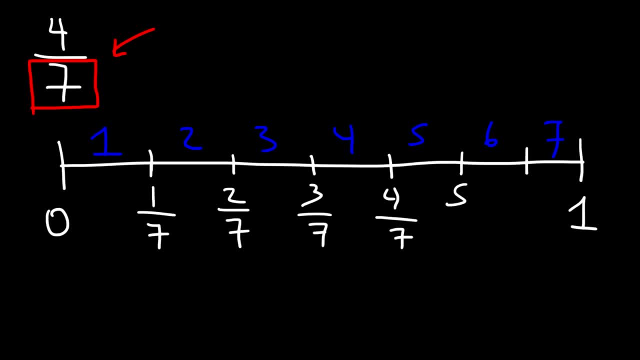 And then you just count it all the way to 7 over 7.. Now, once you get to 1,, 1,, 2,, 3,, 4,, 5,, 6,, 7.. 1 is the same as 7 over 7.. 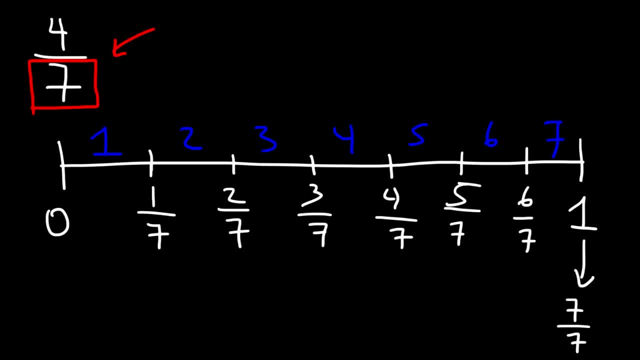 7 divided by 7 is 1.. But now we're looking for the locality of, or the location of, 4 over 7, which is right here. So this is where we should place 4 over 7 along this number line. 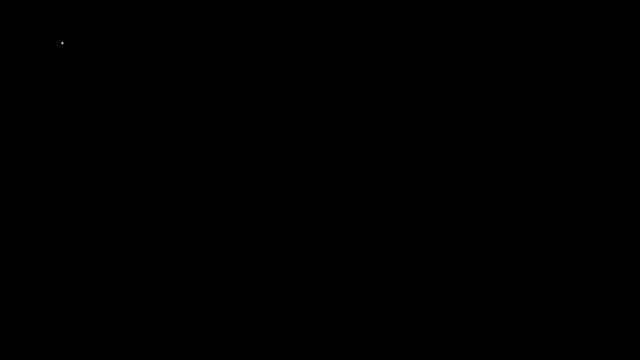 Let's try another problem. Let's say we have the fraction 5 over 6.. Where should we place 5 over 6 on this number line? So feel free to pause the video and try this problem. So let's focus on the number 6.. 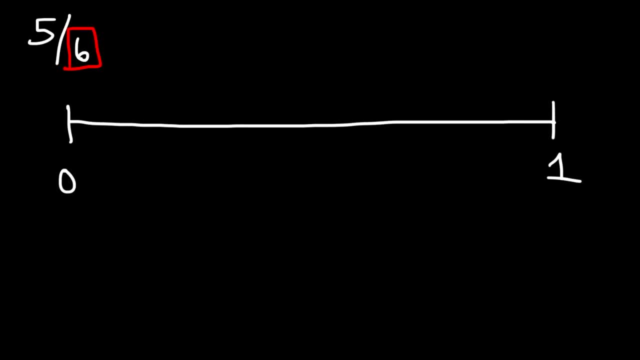 Notice that 6 is an even number, So the first mark I'm going to put is going to be right in the middle. So now I have two equal spaces: One on the left, one on the right. Now I need to break this portion. 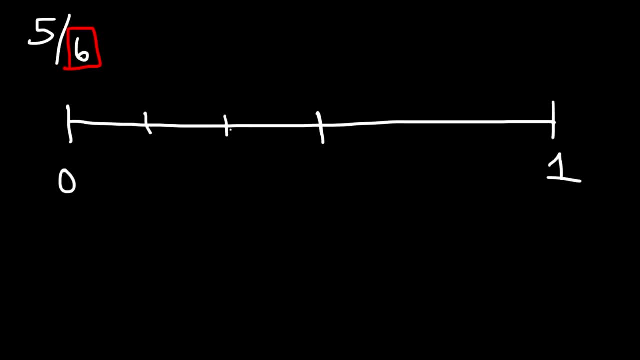 So three equal spaces, So 1,, 2, and 3.. And I'm going to do the same for this side. So now I have a total of 6 equal spaces: 1,, 2,, 3,, 4,, 5,, 6.. 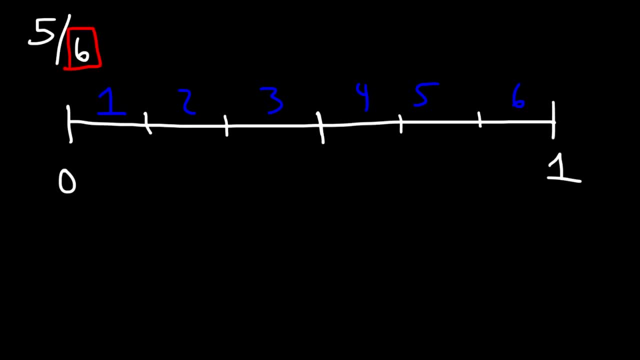 And so I can place the value of the fractions in order. So this is going to be 1 over 6,, 2 over 6,, 3 over 6,, 4 over 6, and 5 over 6. And 1 is going to be 6.. 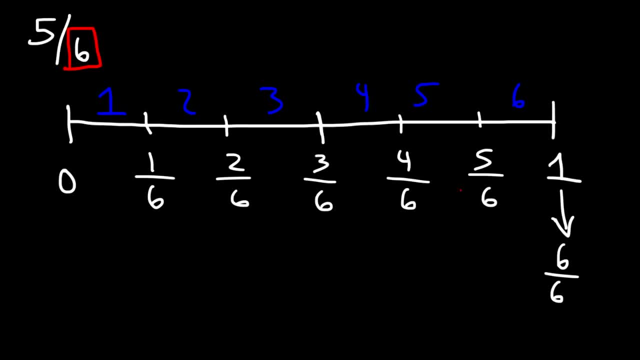 And 6 over 6. And so 5 over 6 is located right here, And so this is where it belongs, along this number line And, as you can see, these problems, they're not that bad As long as you follow the process, if you follow these steps. 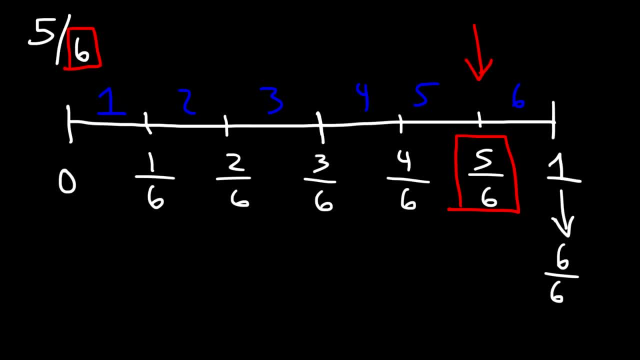 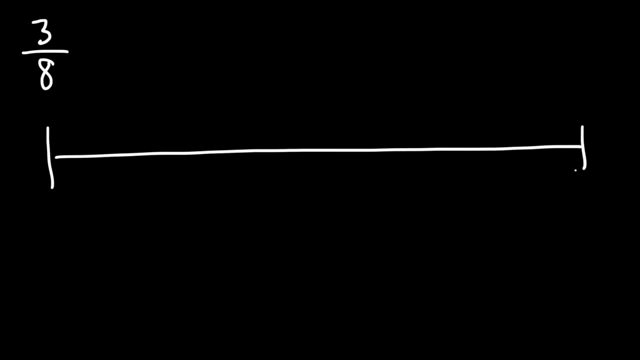 you can easily find where to place the fraction along the number line. Now let's work on one final example: 3 over 8.. If you want to pause the video, feel free. So let's focus on the denominator 8.. 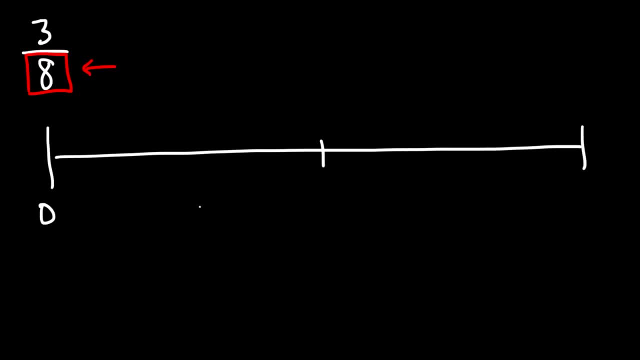 So it's even- I'm going to put a number right in the middle- And so we have 2 equal spaces, And now we have 4.. And now we have 8.. So let's count it to make sure: 1, 2, 3, 4, 5,, 6,, 7..